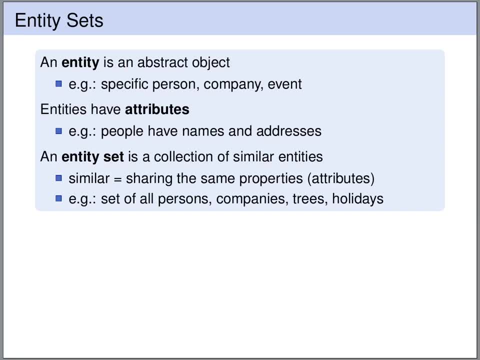 Think, for instance, of a specific person, a specific company or a specific event. Entities have attributes, People have attributes. People have names, addresses, events have a location, a time, a date, and so on. An entity set is a collection of similar entities. 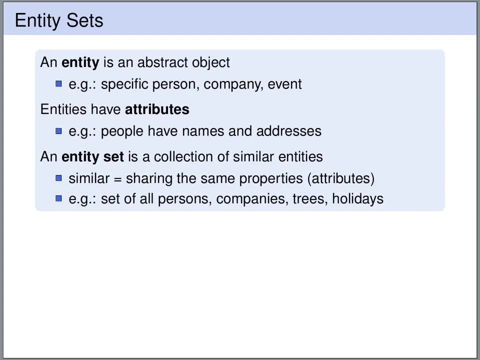 And similar here means they share the same properties, the same attributes. For example, think of the set of all persons, the set of all companies, trees and so on. Again we have an analogy with object-oriented programming. You can think of entities as objects and entity sets as classes. 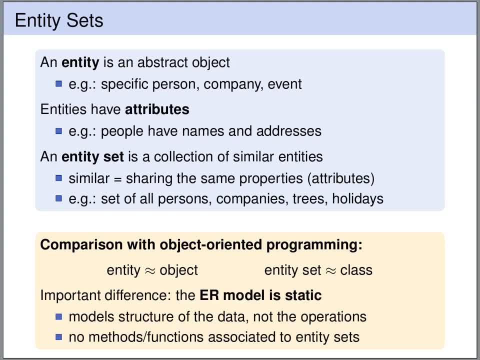 But there's one important difference between object-oriented programming and entity relationship models. In entity relationship models we only model the structure of the data. We do not model the operations. So we do not have any functions or methods associated with the data. In the reality, the data is only associated to entity sets. 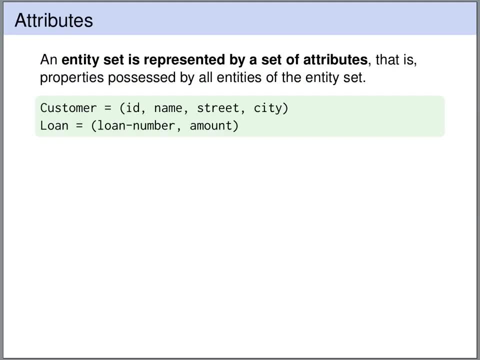 Only attributes. An entity set is represented by a set of attributes that are shared among the entities in this entity set. For instance, every customer entity in the customer entity set has an attribute: ID, name, street and city. Every Loan has a LoanNumber and an Amount. 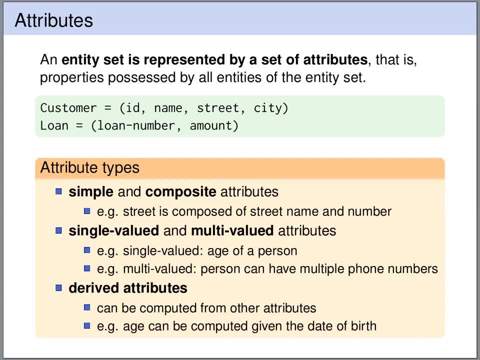 We can have different attribute types and we will see an example on the next slide. We have simple and composite attributes. A composite attribute is composed of many other attributes. For example, a Street is composed of the StreetName and the Number. We can have single-valued and multi-valued attributes. 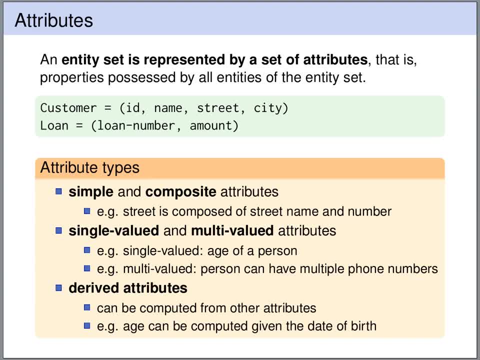 The age of a person is a single-valued attribute. A person has only one age. The phone numbers of a person are a multi-valued attribute. A person can have many phone numbers. We can also have derived attributes. Those attributes can be computed from other attributes. 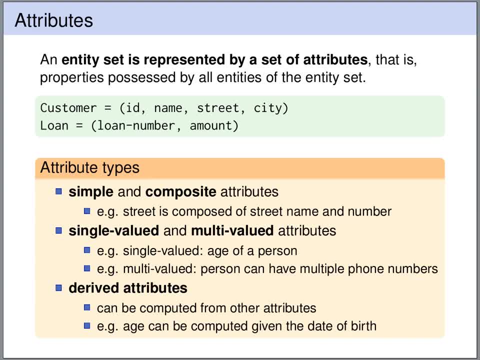 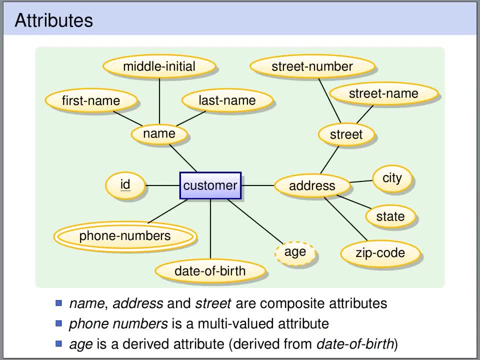 For instance, the age can be computed from the date of birth. Let's look at these different attribute types in an example. The address is a composite attribute. It itself has attributes attached to it. The address consists of the Street, the City, the State and the Zip Code. 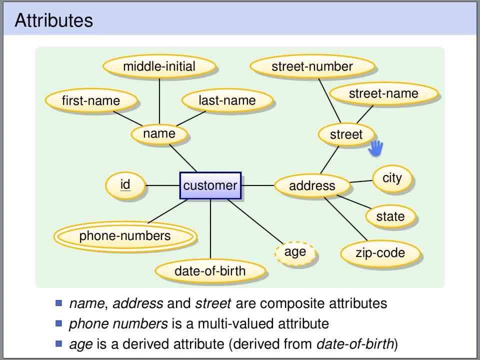 Composite attributes can be nested. The Street is a part of the address and it is itself a composite attribute. It consists of the StreetName and the Number. Likewise, the Name is a composite attribute. It consists of the FirstName, the MiddleInitials and the LastName. 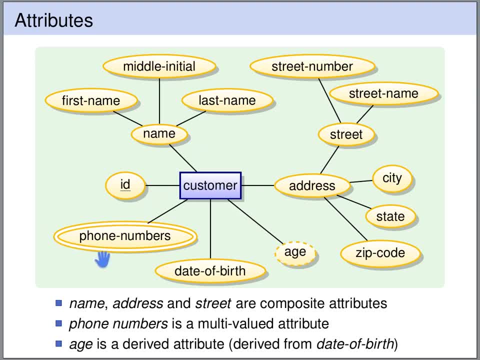 The phone numbers are a multi-valued attribute In the entity relationship diagram. this is indicated by this double line around the ellipse. The age is a derived attribute. It can be computed from the date of birth. Such derived attributes are indicated using a dashed line in the entity relationship diagrams. 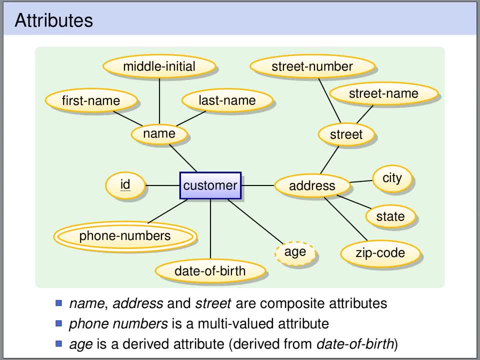 Composite attributes can also be multi-valued. For example, if you want to allow that a customer can have multiple different attributes, then we could make a double line around the address to indicate that this attribute is multi-valued. Let's look at the formal definition of relationship sets. 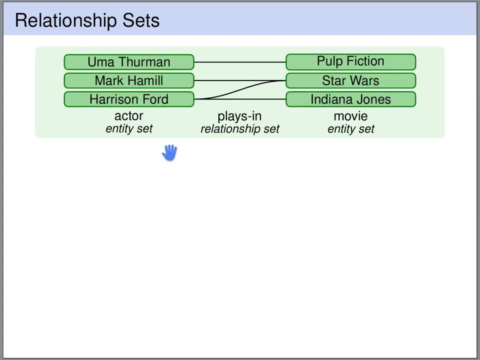 Let's start with an example. Here we have two entity sets. We have an actor entity set which consists of the entities Huma Thurman, Mark Hamill and Harrison Ford, And we have a movie entity set that contains the movies Pulp Fiction, Star Wars and Indiana Jones. 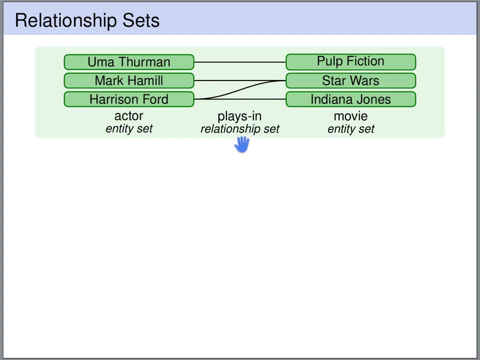 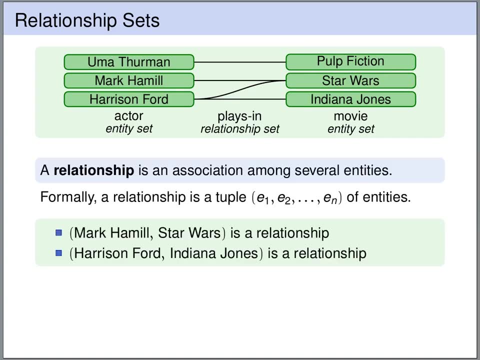 And these two entity sets are connected by a relationship set that is called place-in. A relationship is an association among several entities. Formally, a relationship is a tuple that contains the participating entities. For instance, the place-in relationship set has two participating entity sets. 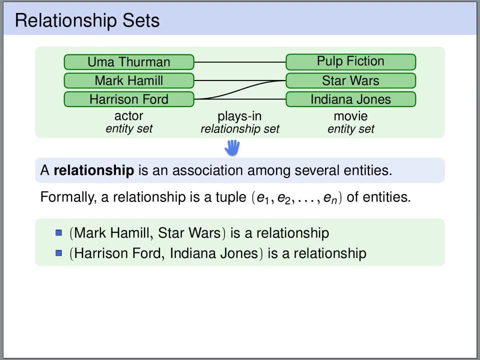 So the relationships in these sets are pairs. These pairs in the example are indicated by these lines. So, for instance, Huma Thurman and Pulp Fiction is a pair in this relationship set. Other examples are Mark Hamill's Star Wars is also a pair. 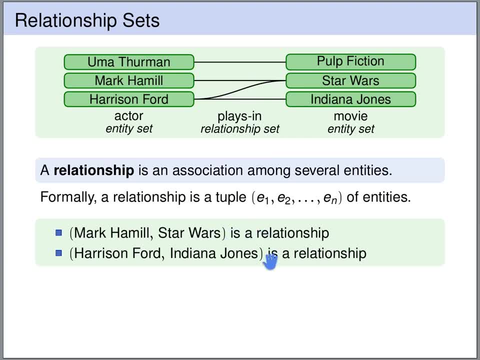 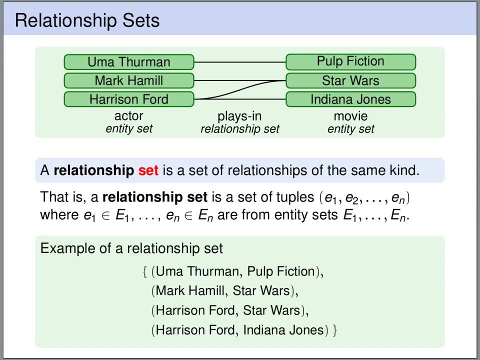 that is in this relationship set, And Harrison Ford and Indiana Jones as well. A relationship set is a set of relationships of the same kind. So formally a relationship set is a set of tuples, e1 up to en, such that e1 is from the first participating entity set. 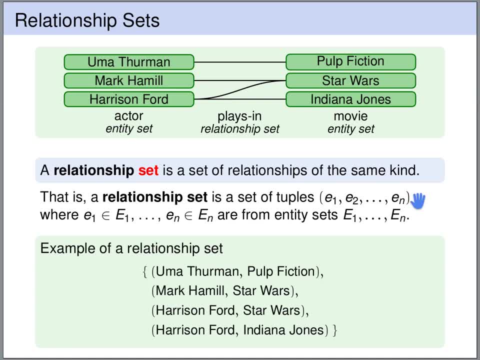 e2 is from the second participating entity set, and so on. The example given above is formally a set of pairs consisting of the pair Huma Thurman-Pulp Fiction, Mark Hamill's Star Wars, Harrison Ford's Star Wars and Harrison Ford-Indiana Jones. 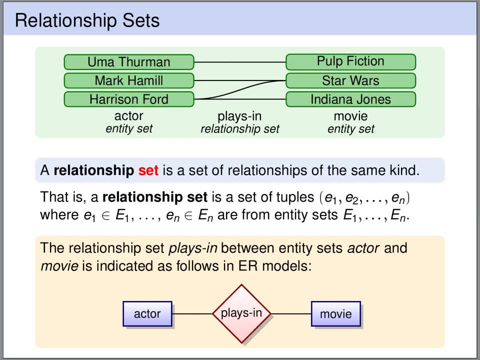 In the entity relationship diagrams the relationship set place-in between the entity sets Actor and Movie is indicated using the diamond And it is connected using lines to the Actor entity set and to the Movie entity set. To improve readability, we can annotate the connections. 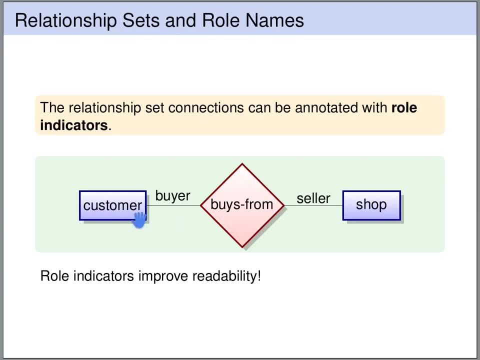 between the relationship set and the participating entity sets with role indicators. So in this example we have an entity set Customer and an entity set Shop and they are related by a buys-from relationship set. Here we can annotate the connection to the Customer with the role Buyer. 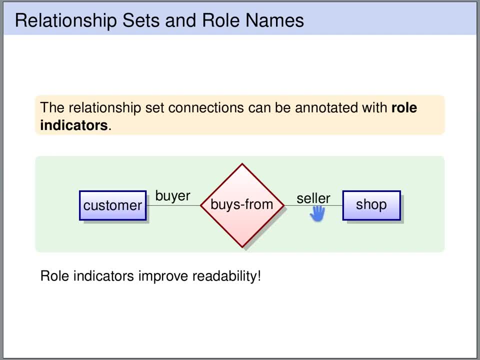 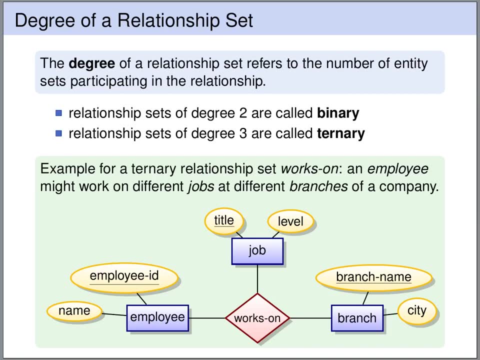 and the connection to the Shop with the role Seller. The degree of a relationship set is the number of participating entity sets. A relationship set of degree 2 is called binary. A relationship set of degree 3 is called ternary. Up to now we have only seen 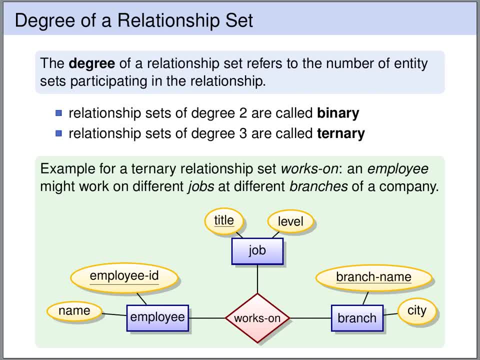 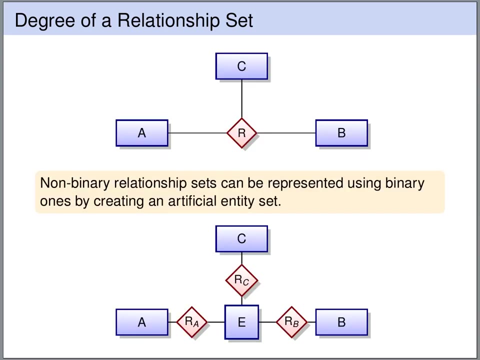 binary relationship sets. On this slide we have seen an example of a ternary relationship set. Here we have a ternary relationship set works on. It is used to express that an employee can work on different jobs at different branches of the company. Strictly speaking,